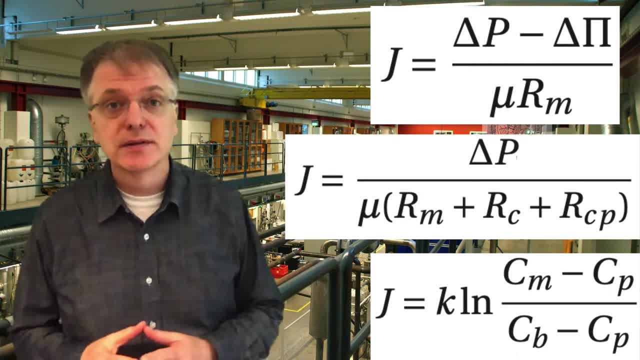 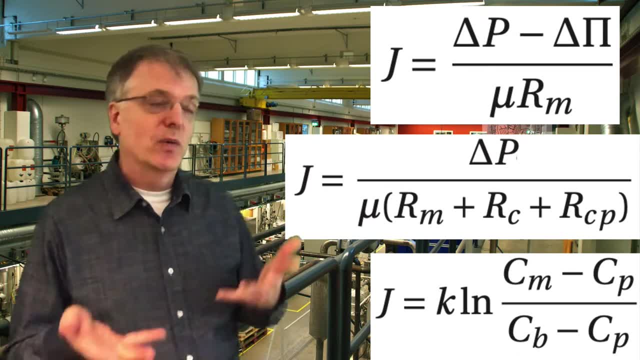 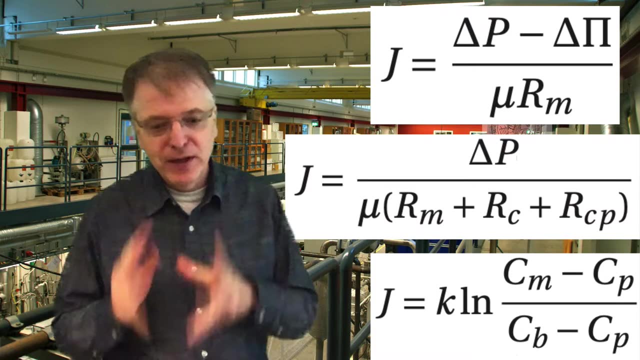 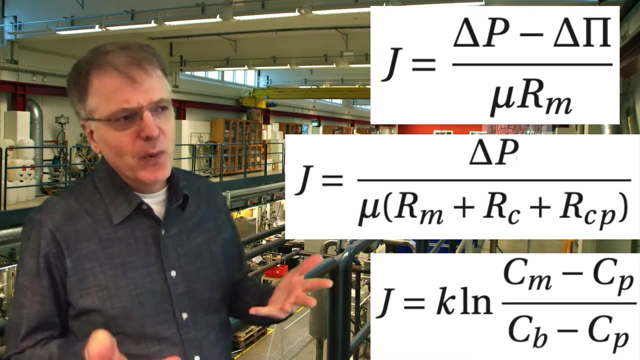 We use these three models for membrane filtration in our course separation processes And since students ask when should I use which model, I made this video to try to clarify these things. Now, the thing is that all these three models are simplifications. And when should you? 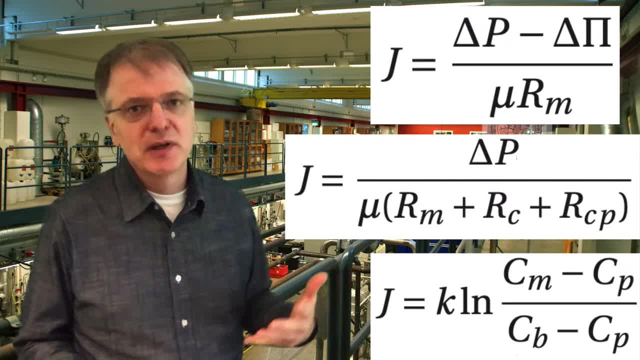 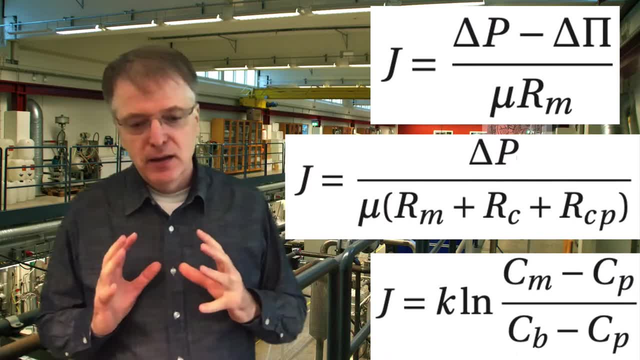 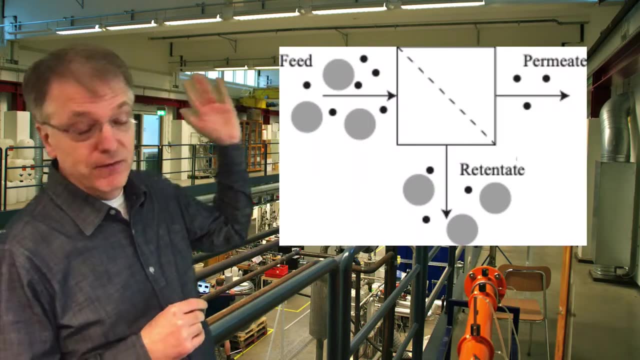 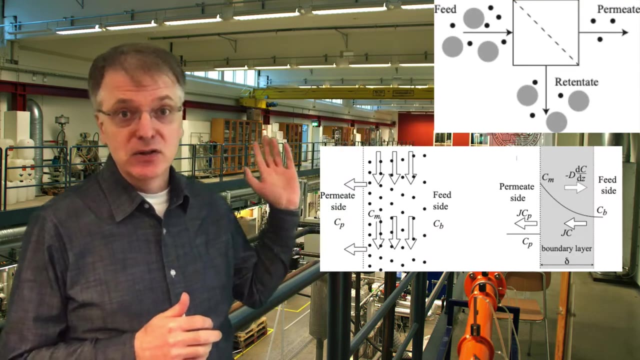 use which, Well, it depends on what you can assume to be negligible. And all these three are simplifications. So what is the situation when you do membrane filtration? Well, you have a feed coming in and you have a retentate going out and a permeate going out. On the feed side, you have a 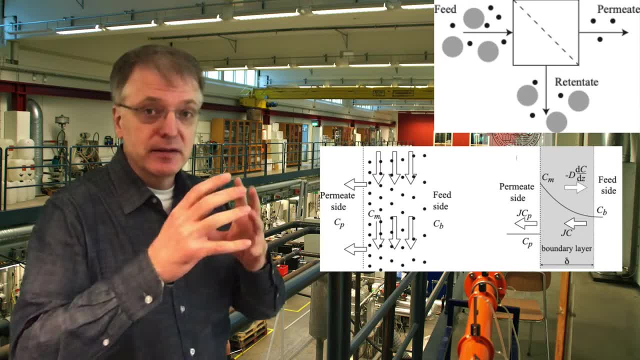 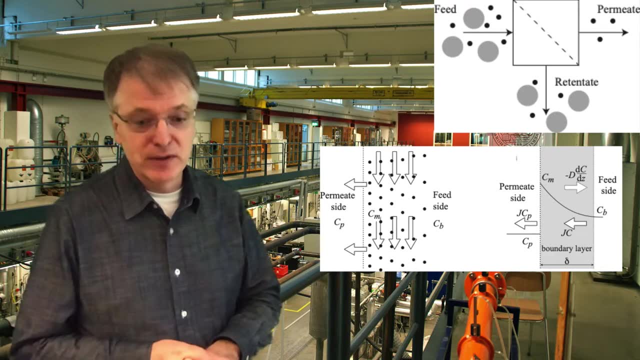 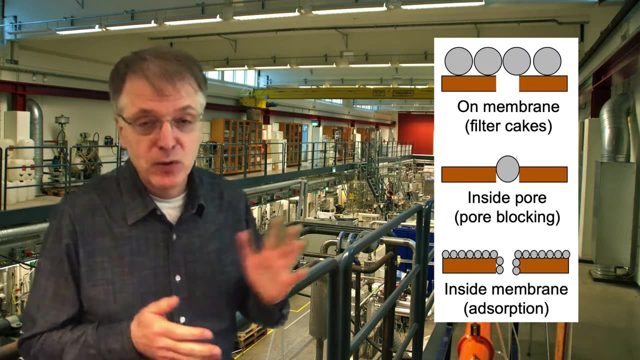 certain concentration in the bulk of the solution, but at the membrane surface you typically have a higher concentration. and then in the permeate you have a third concentration right. Another thing: if you looked at closely at the membrane, you might have fouling on the membrane. 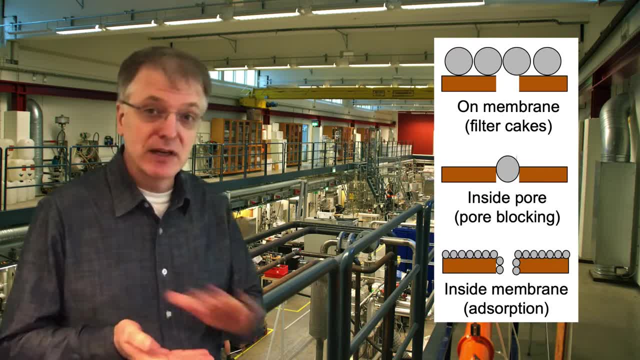 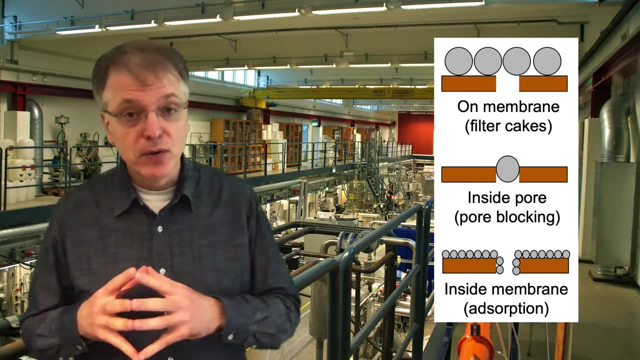 or you typically have some kind of fouling and you might even have a cake forming at the membrane and you might need to take that into account. So if, for example, you have a situation where the bulk concentration is a little bit higher than the membrane surface, then you might need to. 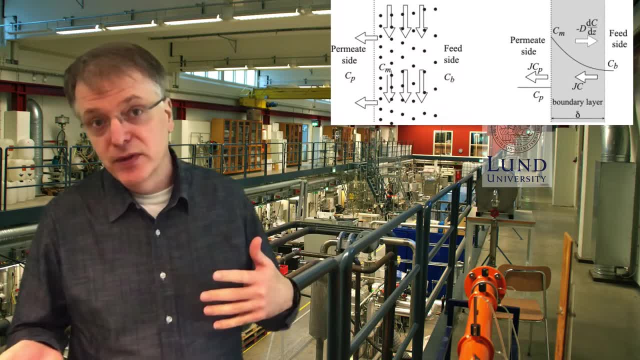 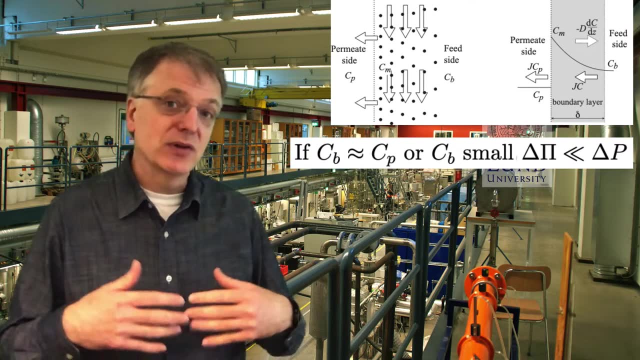 use a salt binder. But then, basically, what would happen if the montane concentration should be more than the permeate concentration, or if the solute concentration is very similar to the permeate concentration? Well then, there is not much of a difference in osmotic pressure And the same if concentrations. 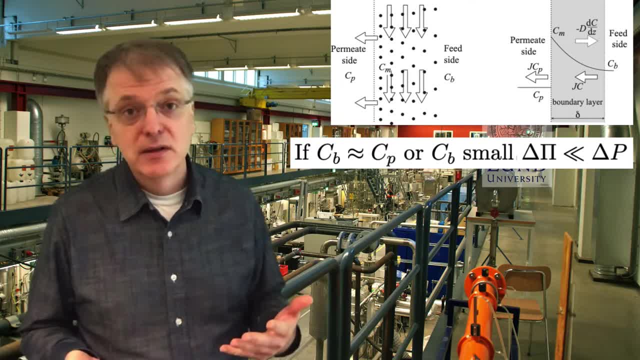 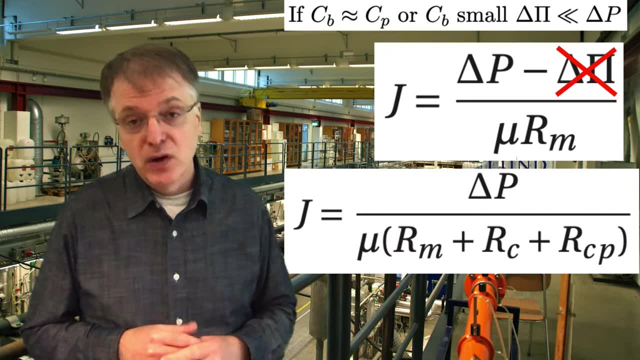 are low than the osmotic pressure is low anyway. So then you don't need to take the osmotic pressure difference into account. And could this be the case? Well, for example, if youות desalt proteins, We can't concentrate proteins to very high station energy and they might put 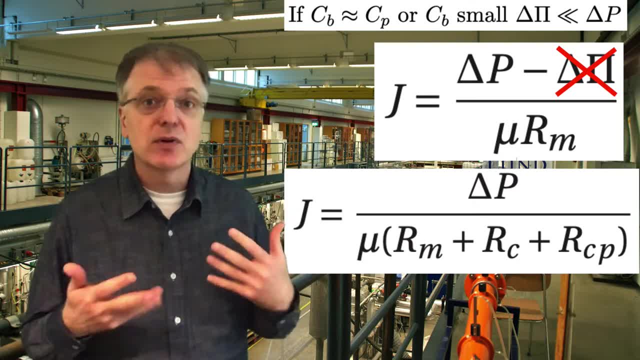 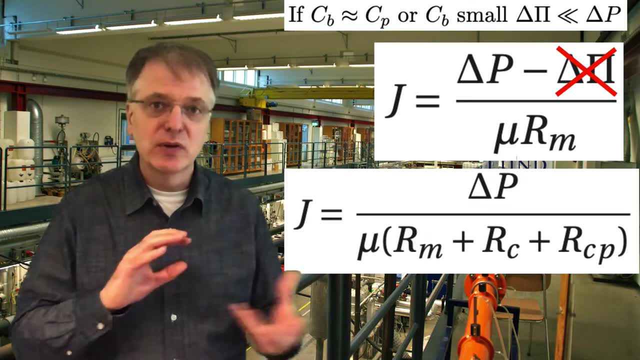 thousands of Н or N breaking out of the京, deserved by a completely liquid function. As you can see, we concentrate proteins to very high concentrations because they are so big and bulky. so they might- Yeah, they might be destroyed. They might clog together to bigger agglomerates of several proteins together. 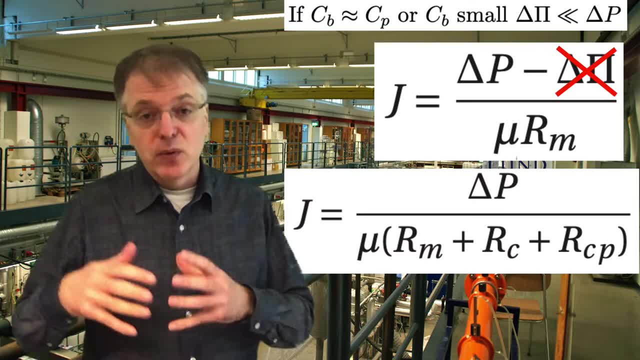 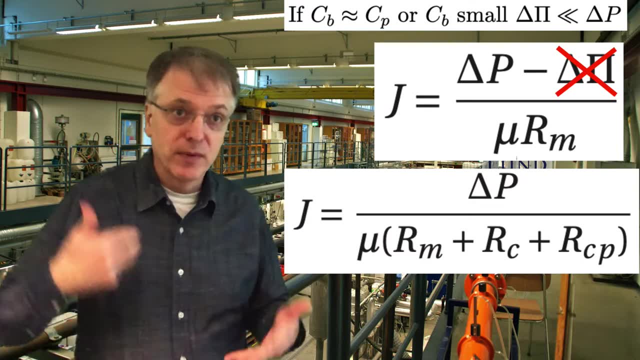 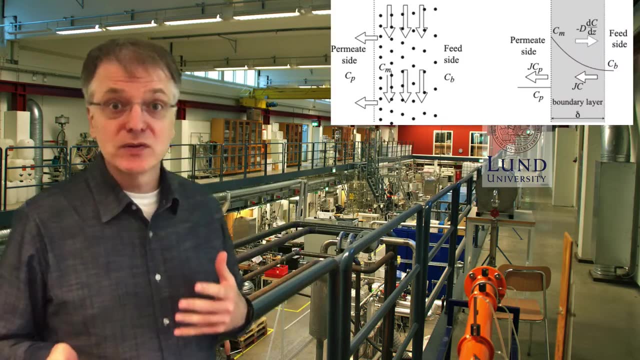 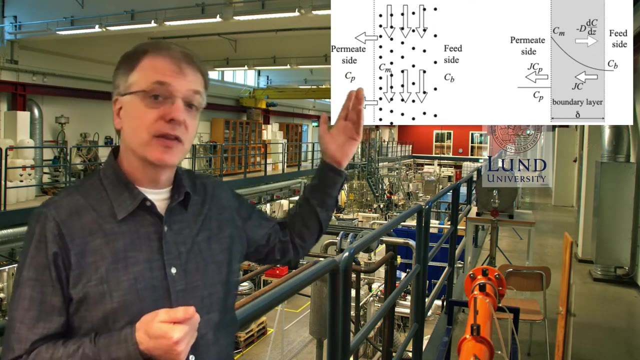 several protein molecules. So then you can often assume that the osmotic pressure difference on the two sides- on the feed side and the permeate side- is negligible. furthermore, if you have low concentrations, then the difference between the bulk concentration on the feed side and concentration and the membrane surface 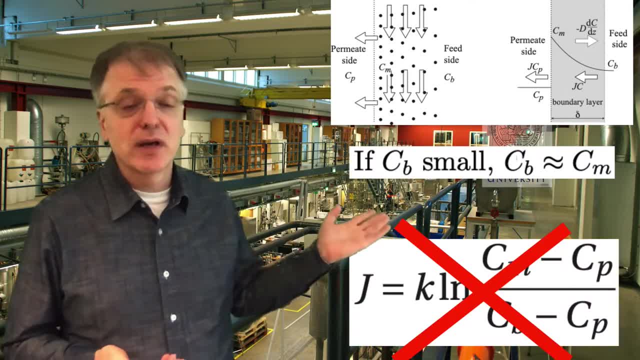 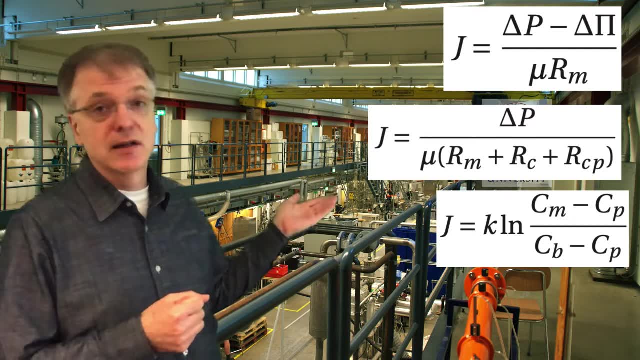 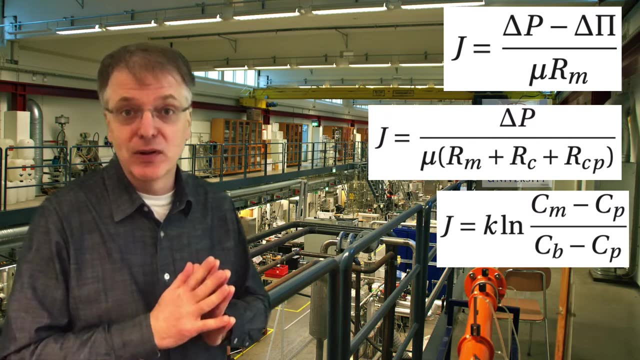 will be Negligible. so then you can say that, okay, Concentration polarization is not an issue. So if we go back to these three models, then clearly, if you have no concentration polarization to talk of, then Yeah, you can't use the concentration polarization model, right? 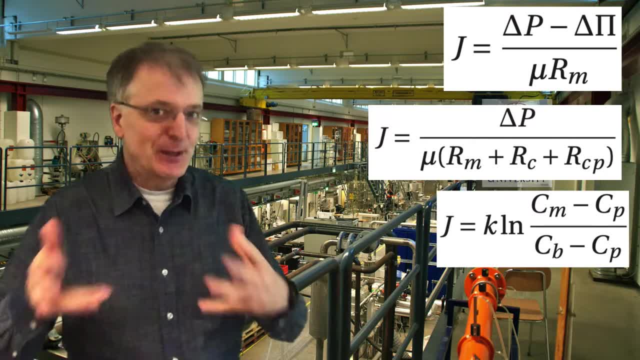 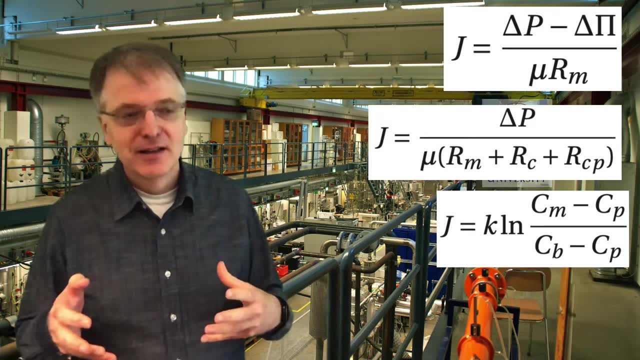 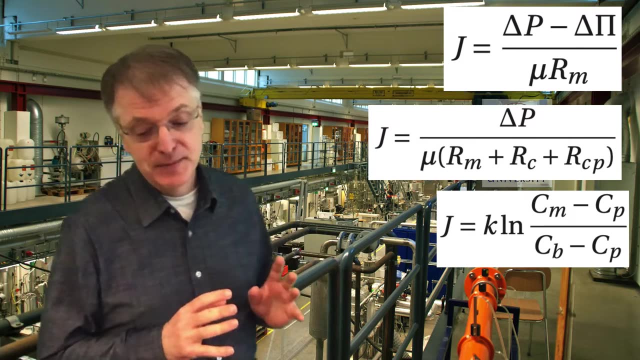 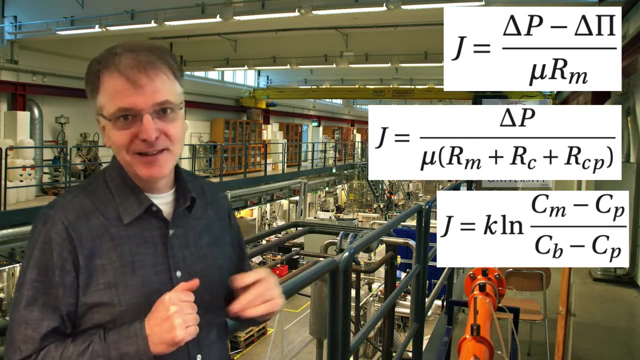 but Unfortunately typically we do Okay, because typically we want to concentrate stuff and as soon as we do that There will likely be a concentration difference between the bulk and the membrane surface on the feed side. so you see, in the Resistance in series model there is an RCP which is 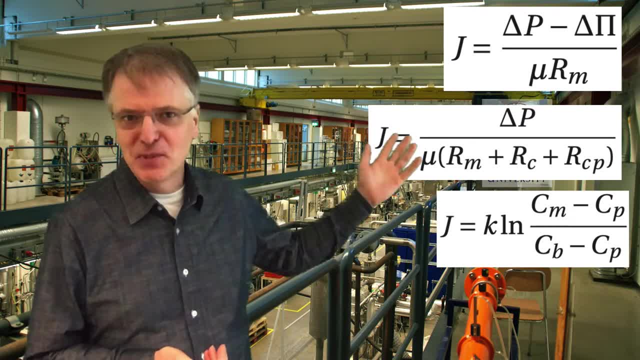 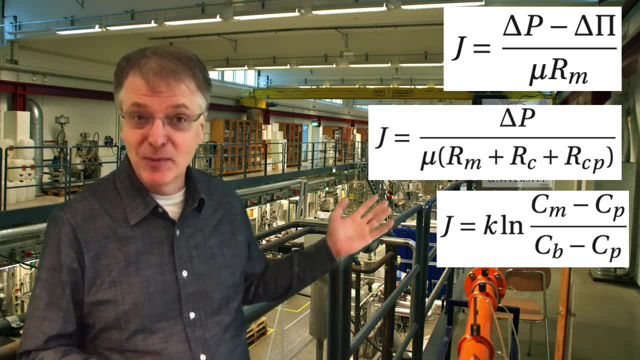 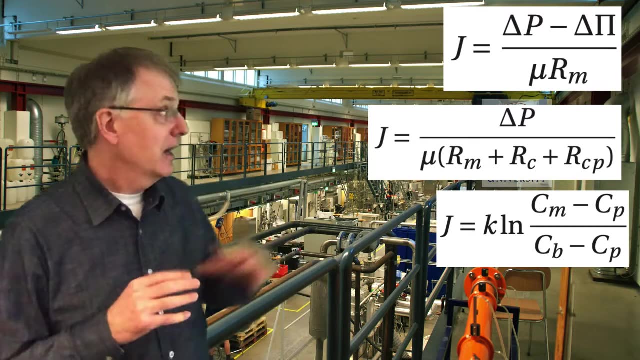 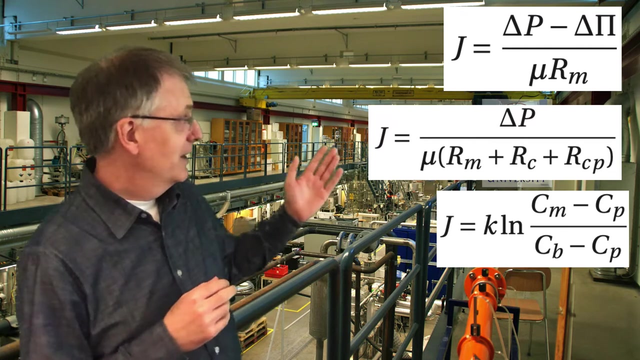 Concentration polarization resistance just as a number. so you have somehow, you have to get to that number, either by using the concentration polarization model somehow or doing some measurements, which might not be very straightforward. and if you look at the resistance in series model, well, in the way we have written here, there are three resistances: the resistance in the membrane, as 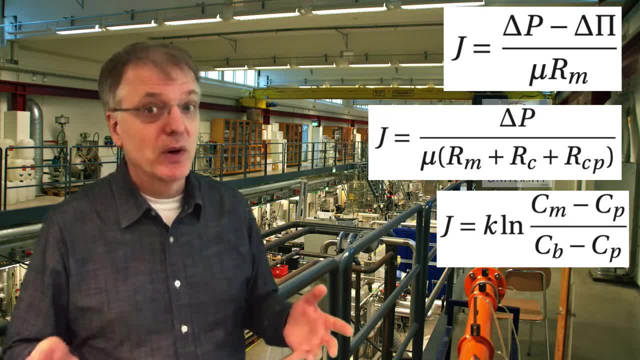 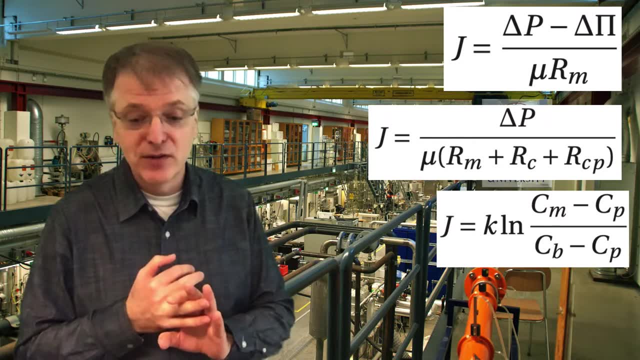 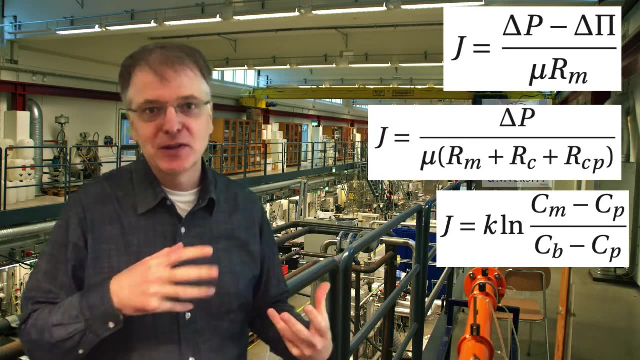 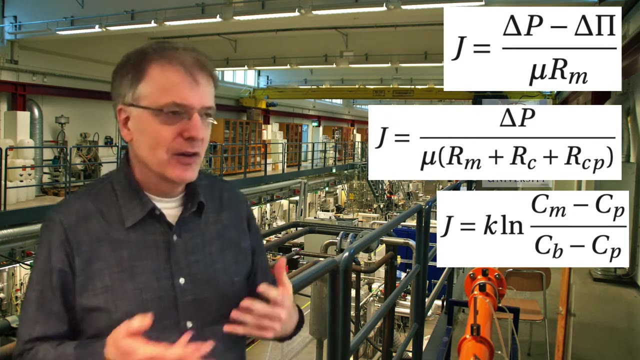 such, and then two others, but there might be more. so cake resistance is one thing and other kinds of fouling is another thing, but you could think of adding osmotic pressure resistance as well, but then you need to determine all these resistances somehow, and the only one that 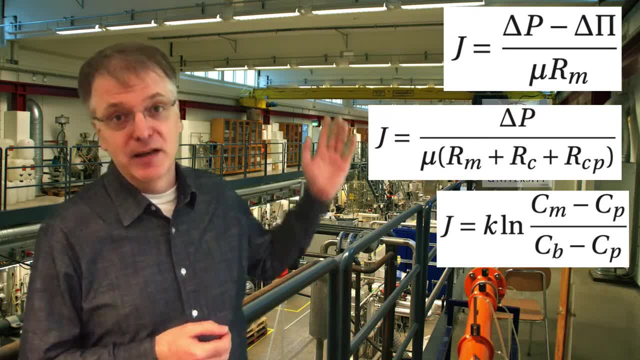 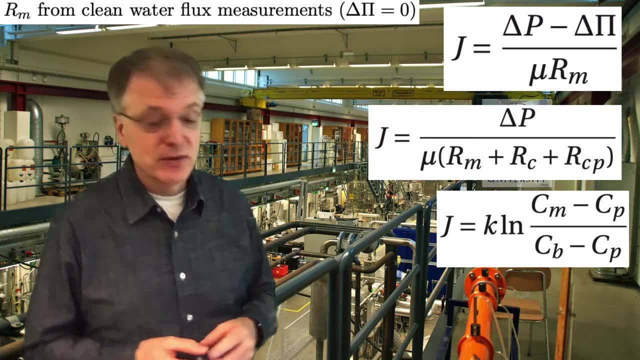 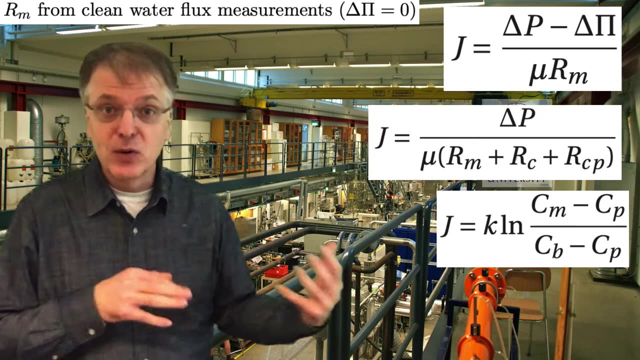 is straightforward to determine is the membrane as such, the membrane resistance, because that you can do with clean water flux, also called pure water flux, because if you look at the first model here, if you have clean water the pi thing goes away, because there is no difference. osmotic pressure: because there is no osmotic pressure, because the concentration is zero. 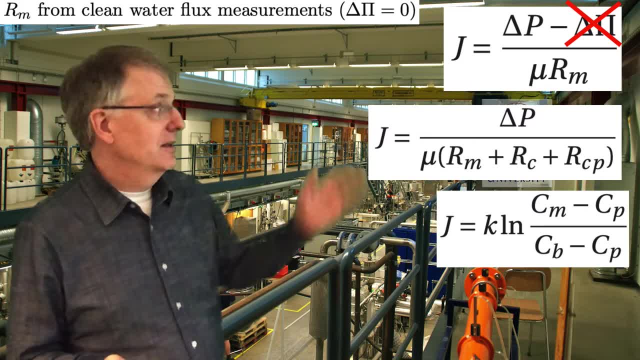 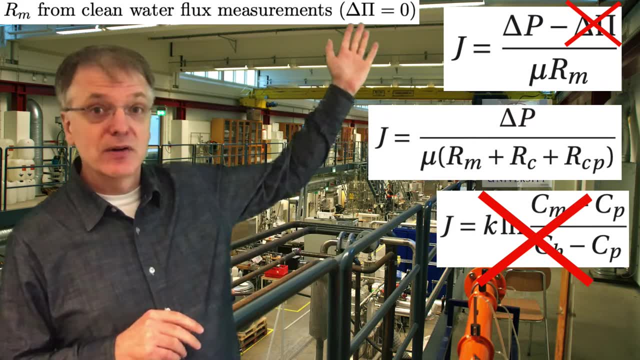 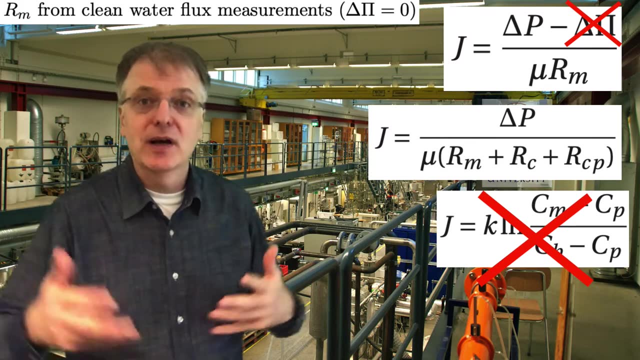 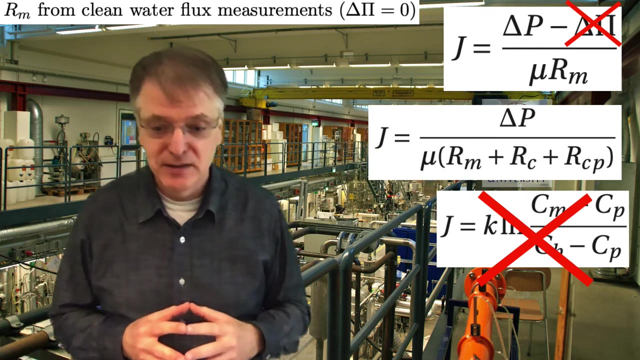 you only have water, and yeah, and if you have zero concentration, then the concentration polarization model is not to be used, right? so then you can use this: first the osmotic pressure model to calculate rm, and then you have that, and then in the resistance in series model you need to somehow determine the other resistances. 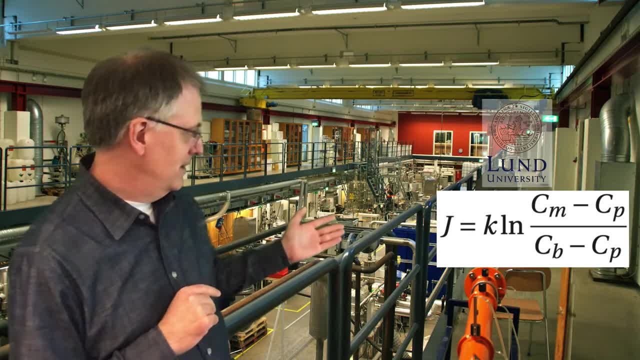 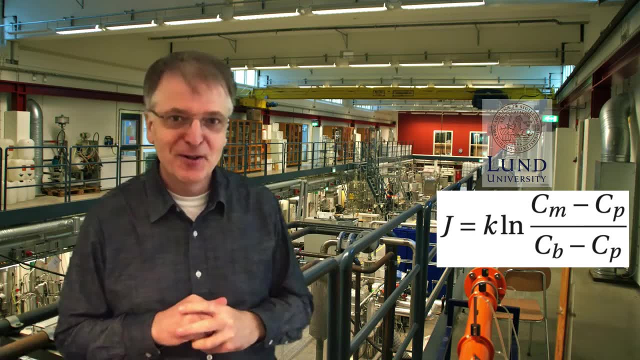 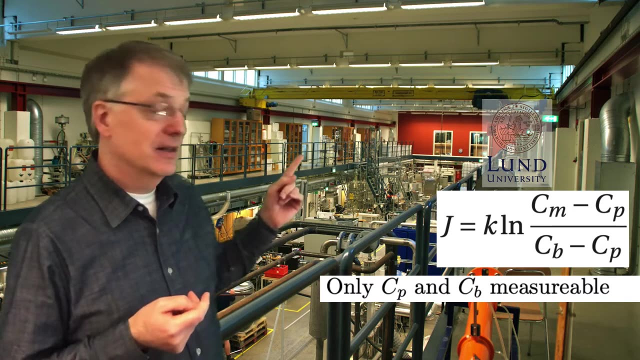 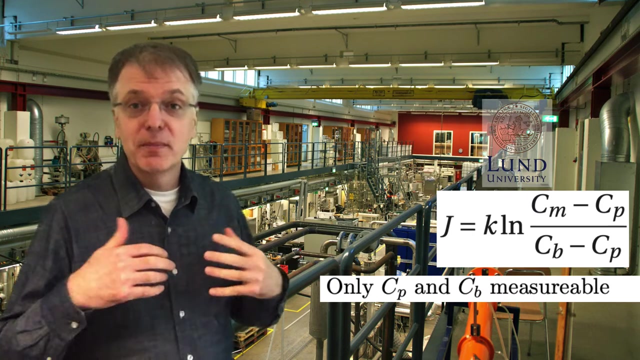 okay, a problem here is that the concentration polarization model seems simple enough, but there are two very tricky things here. firstly, the only two concentrations you can actually measure is the concentration in the bulk on the feed side and the concentration in the permeate, the concentration on the membrane, at the membrane. 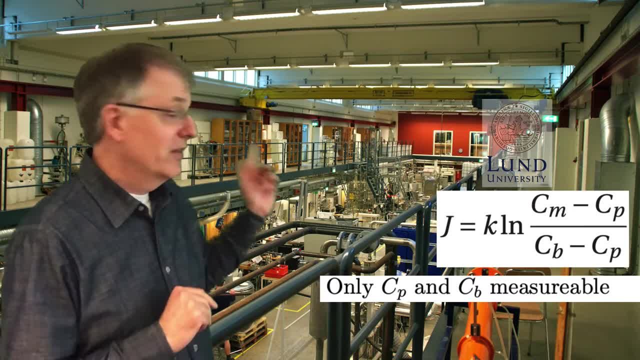 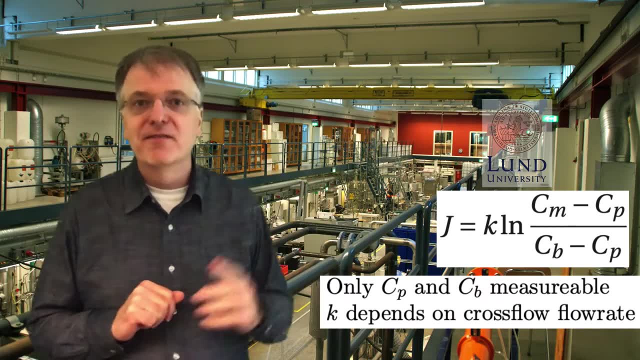 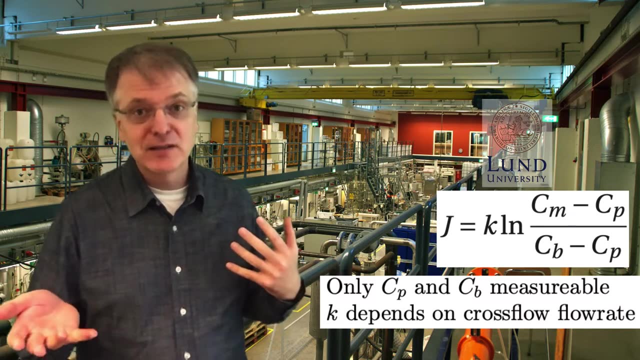 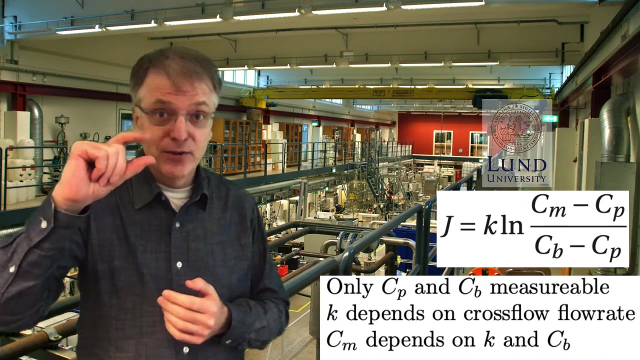 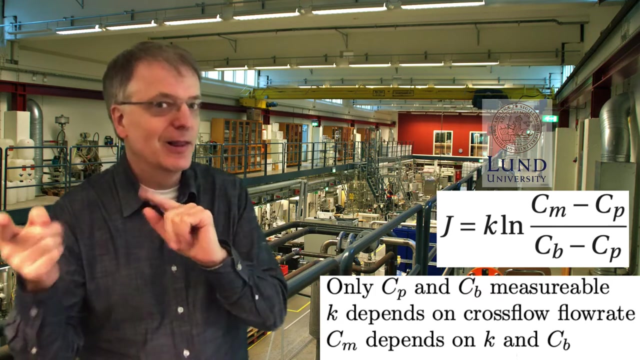 surface, you can't determine. furthermore, there is a mass transfer coefficient here, k, and that mass transfer coefficient varies with circumstances. so the higher the cross flow rate is, the higher the mass transfer coefficient. but the higher the mass the cross flow flow rate is, the thinner the boundary layer will be and hence the lower the difference between the concentration at the. 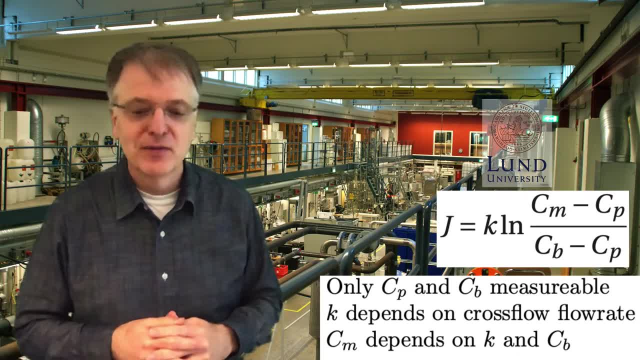 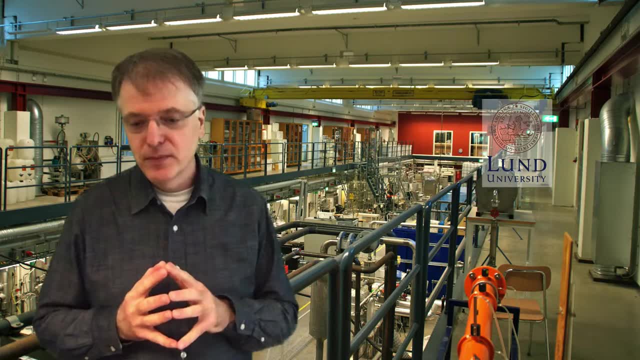 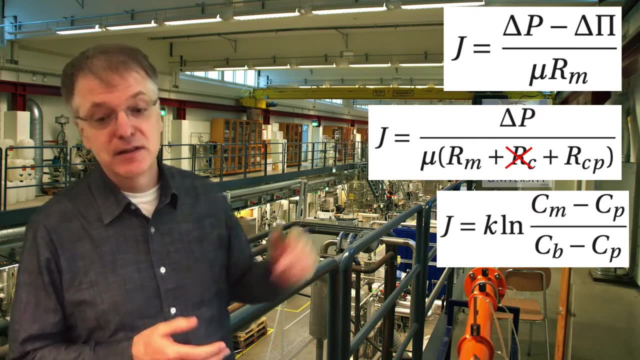 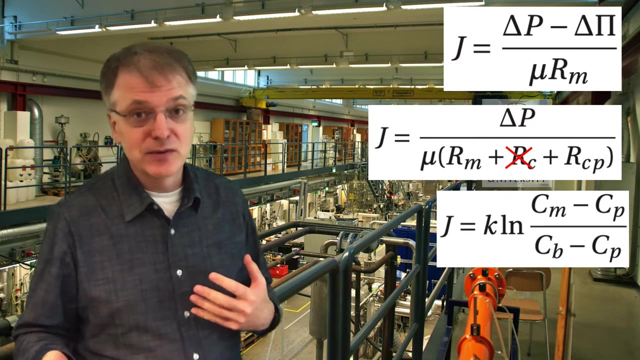 membrane surface and the bulk on the feed side. so this is a bit difficult. so you need to think of what can i neglect? if there is no cake forming, then the rc here and the resistance and series model goes away. if there is no fouling, and then there is no resistance according to fouling. note that in. 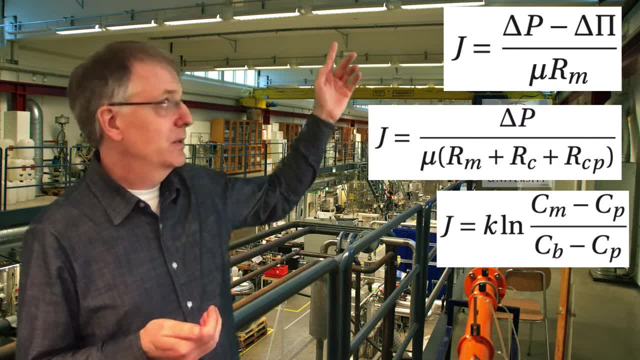 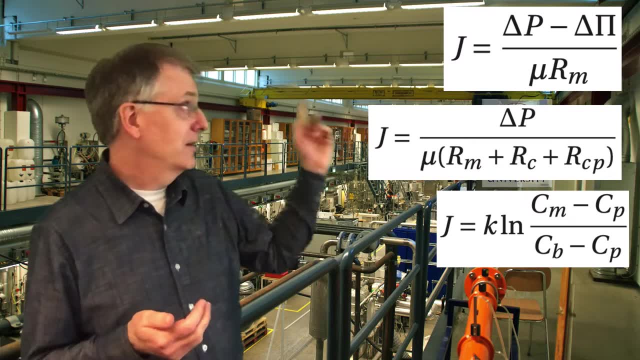 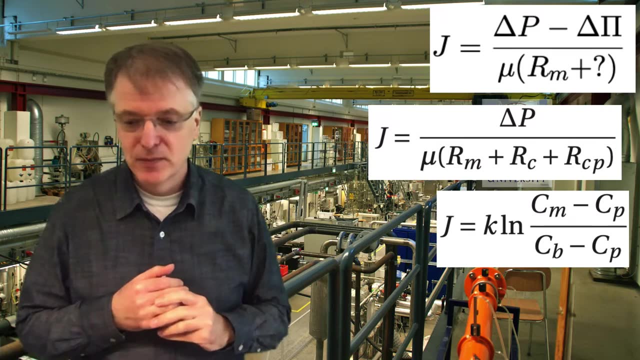 the osmotic pressure model we have up here. we didn't include following, but you could actually combine these two and say that, well, you take the viscosity times rm plus r, following, for example, in the osmotic pressure model, and you can combine these two and say, well, you take the velocity times r and in the osmotic pressure model. 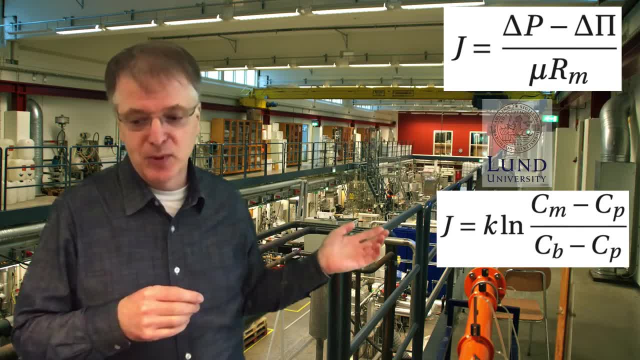 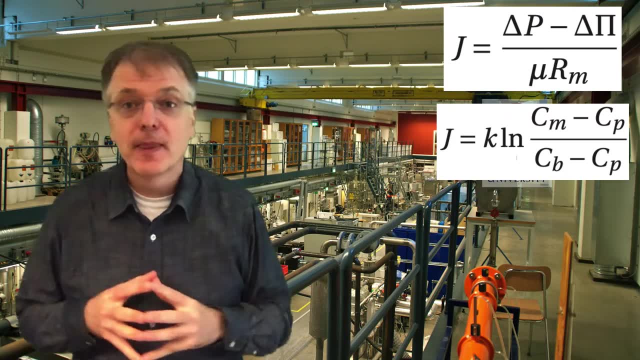 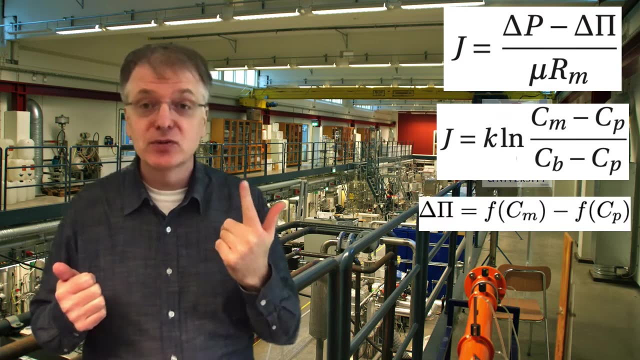 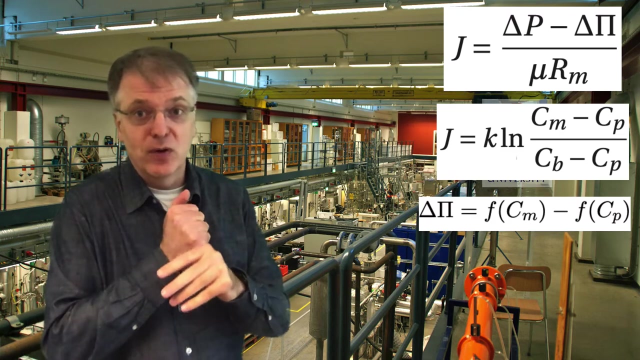 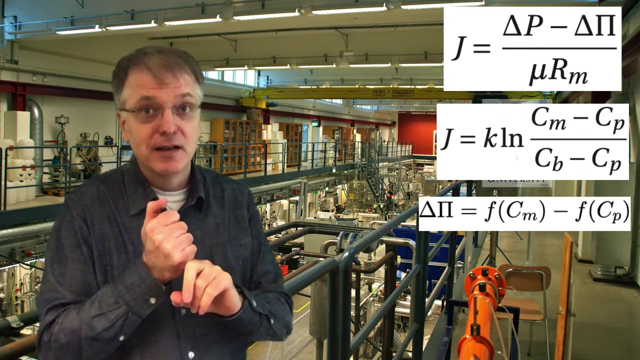 and refuel, and that's the first and the third near the membrane surface. so the osmotic pressure on the feed side is a function of the concentration at the membrane surface, cm, and osmotic pressure on the permeate side is a function of cp. 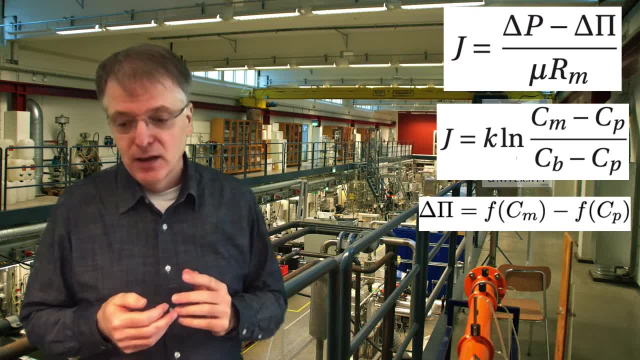 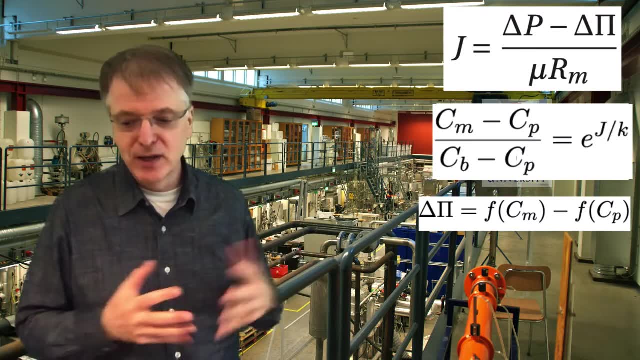 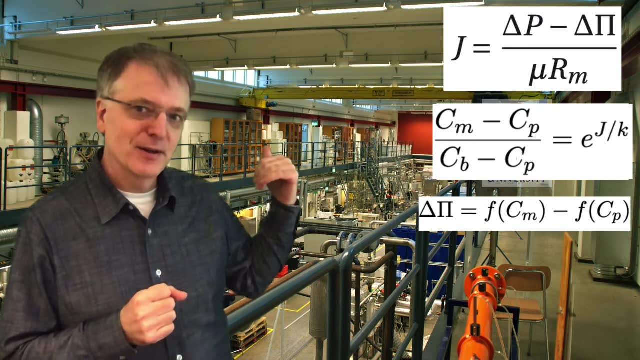 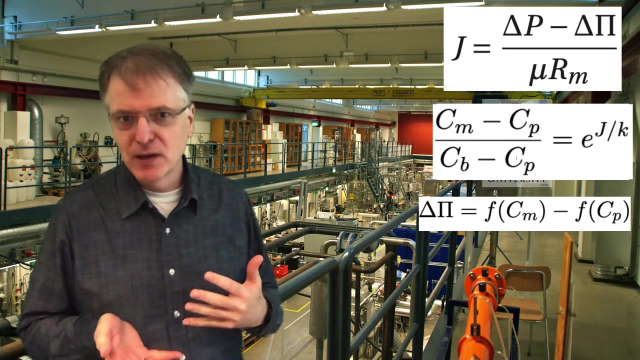 concentration in the permeate. okay. but if we look at the concentration polarization model and reshuffle that a bit, we see that, yeah, okay, now there is some relation here between cm, cp and cb and and the flux through the system and the mass transfer coefficient. we need some more equations. well, perhaps we can come up with an equation that tells: 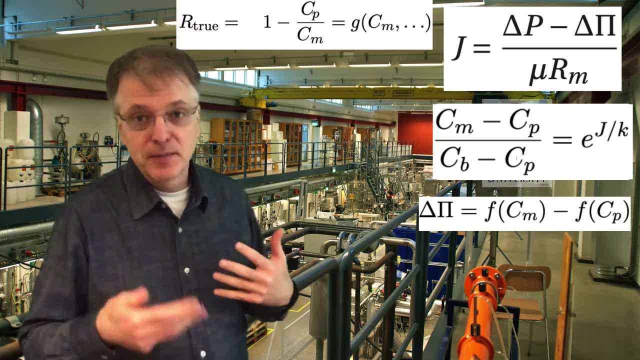 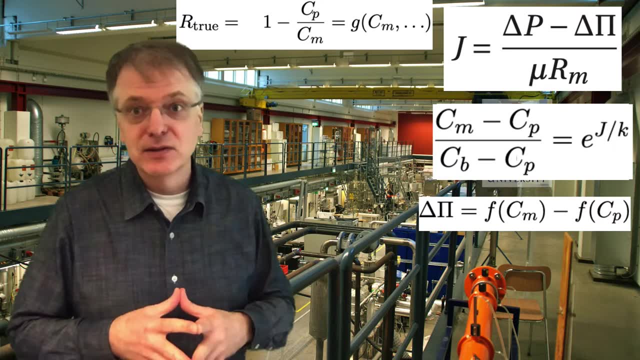 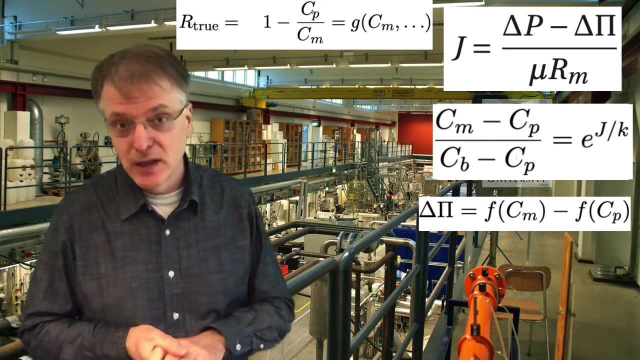 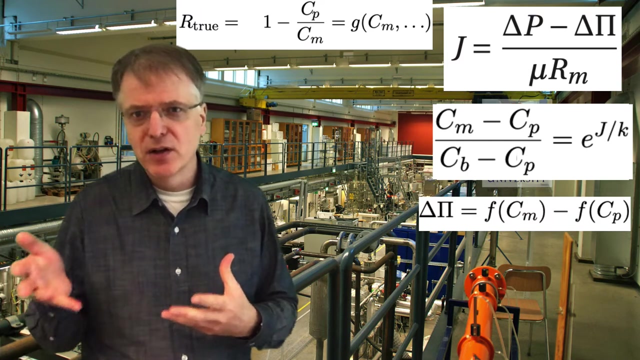 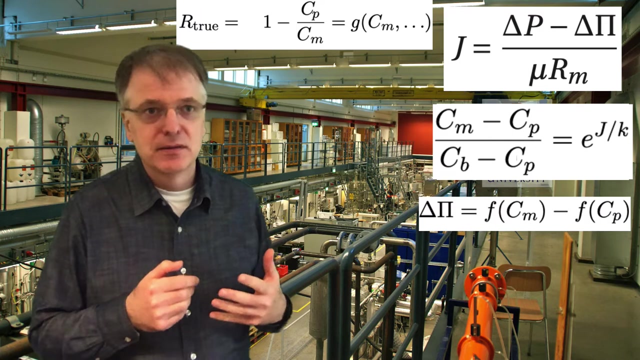 us something about the retention, so some kind of function that gives us the retention given, cm and cp, for example, or the- probably also the cross flow flow rate, right, and then we might be able to combine these somehow. the problem is that there won't be an analytical solution typically, so you have to stuff all this into a computer and try to find a. 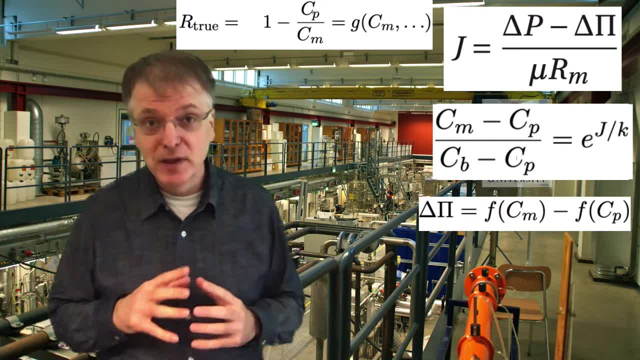 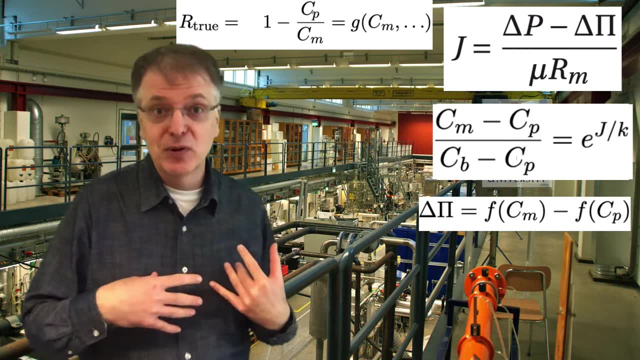 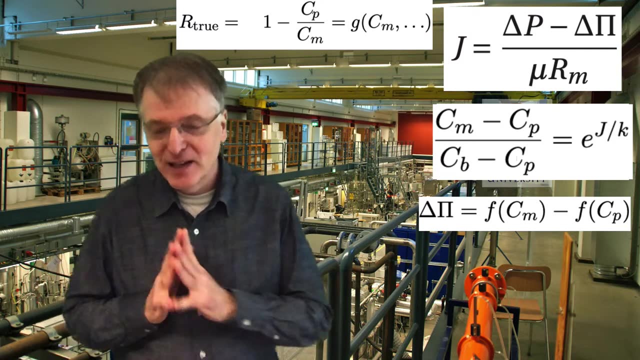 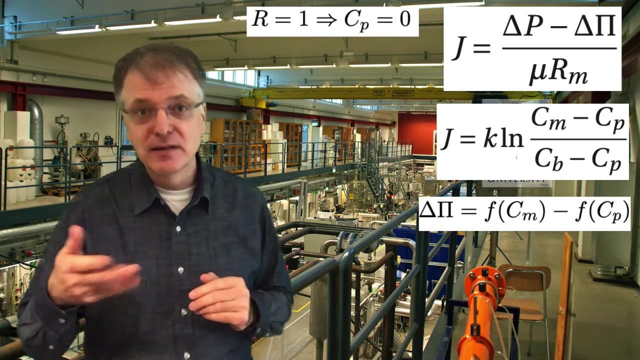 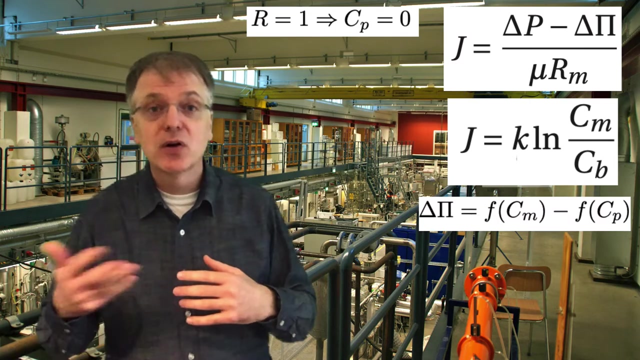 solution. but there is one possibility: when things simplify and you can combine the osmotic pressure model with the concentration polarization model and get something rather simple but still a bit tricky. so if we say that the retention is 100 percent, then cp is zero, then the reshuffled concentration polarization model simplifies and we can calculate the. 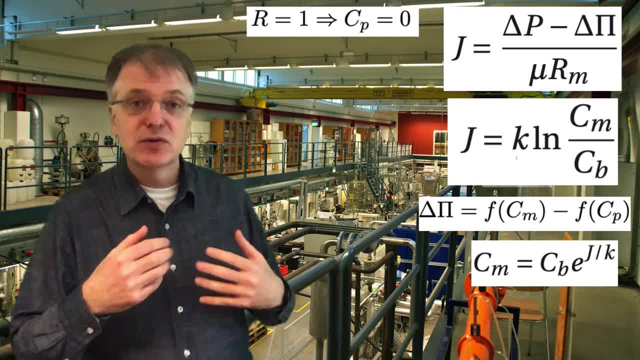 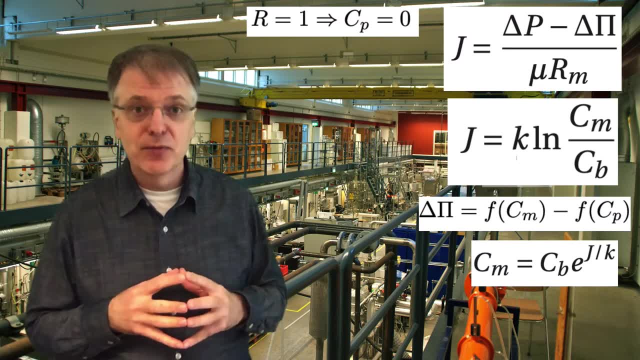 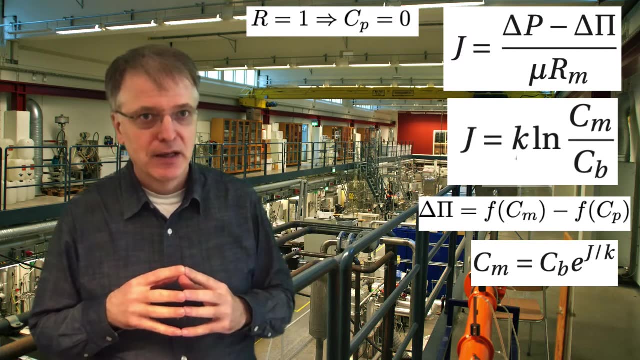 concentration at the membrane surface, from the concentration in the bulk times e to the power of the flux divided with the mass transfer coefficient. well, there is a problem here, right, because we need to know the mass transfer coefficient. but if we, if we have a way to do that, then we can take this thing here.